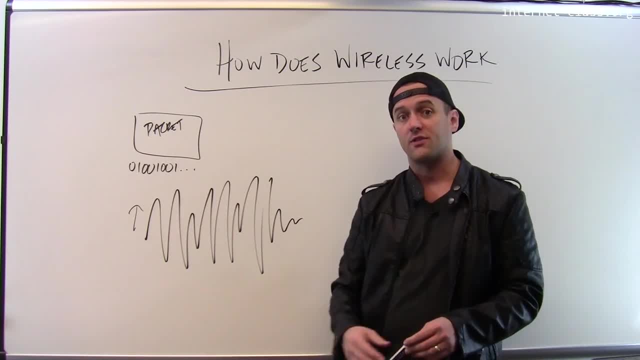 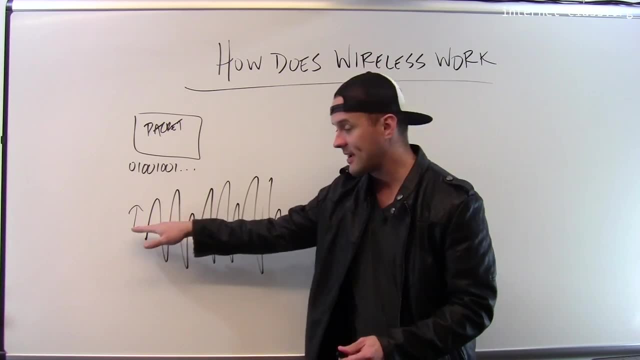 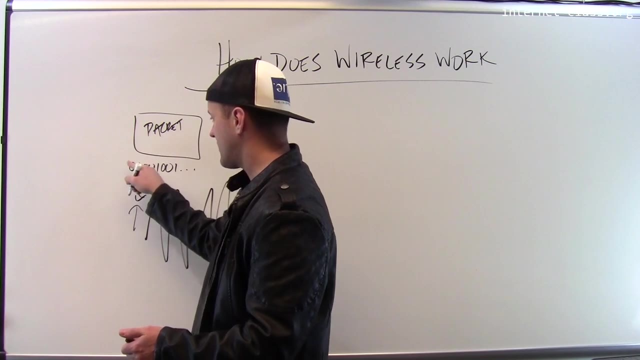 that I'm expecting. So if I need to send data over a kilometer versus 100 meters, the encoding techniques may vary, But these are the fundamentals. What I can vary at the signal level is amplitude and frequency, So I convert this And again this process right here. this one arrow is something that 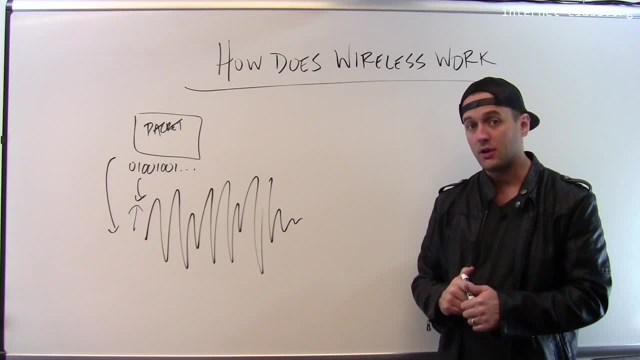 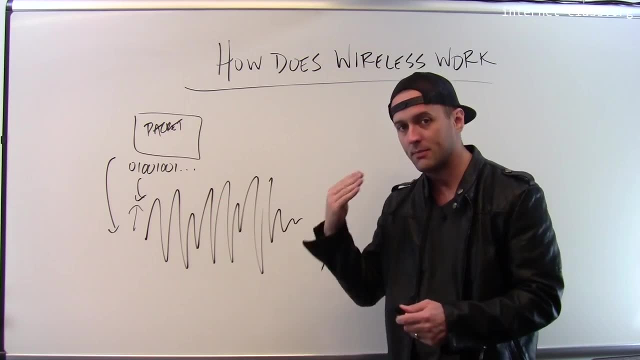 you could talk about for weeks, And if you learned exactly how that worked, you would know a lot about how computers work and about how wireless works. So this signal gets, And so this signal is transmitted by the device that is trying to send data. So it has a radio. 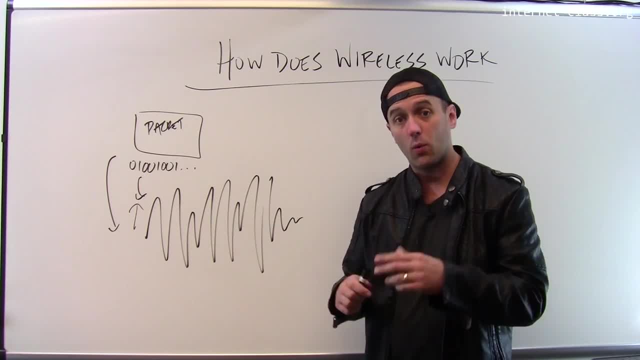 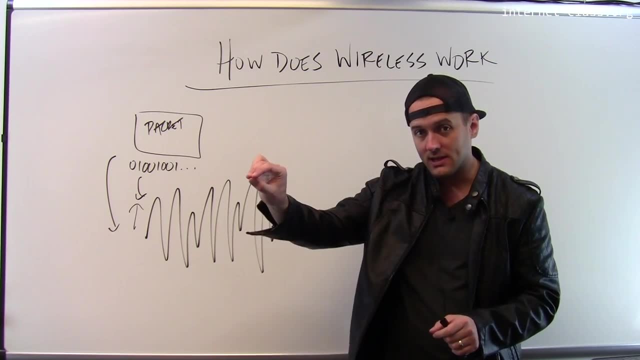 on it and that radio broadcasts a signal. Wireless is fundamentally unlike wires. wireless is fundamentally a broadcast medium. I can do things to direct the signal through antennas, but that signal is going to propagate in free space And even if I try to point it very, 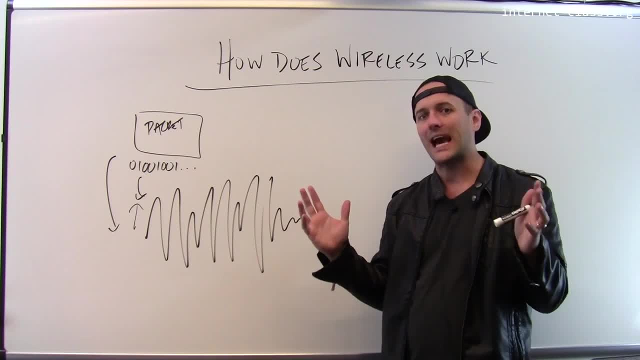 directly in one particular direction, there's still parts of it that are going to leak out into other areas. So to transmit a packet, I have to take the series of ones and zeroes and I have to transmit the signal to the device that is trying to send data, And so this signal is transmitted. 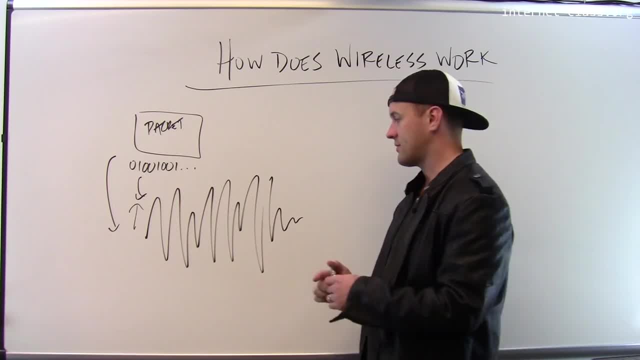 by the device that is trying to send data. So it has a radio on it and that radio broadcasts a signal and that data is going to propagate in free space. So this signal is going to propagate in free space. I have to transmit the signal to the receiver and the receiver 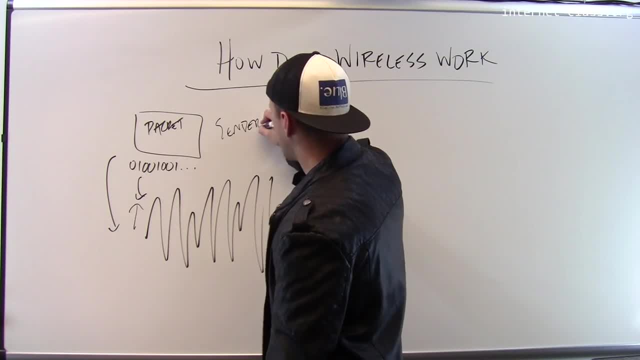 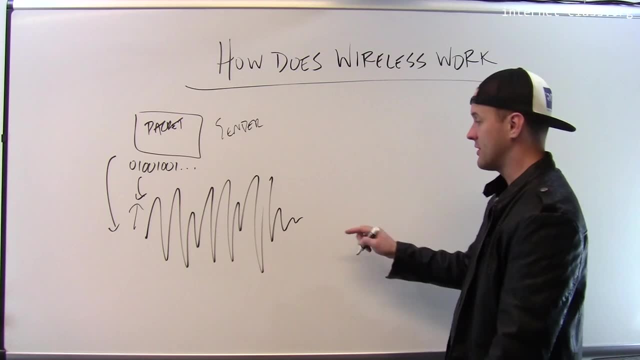 has to have a receiver that is trying to send the signal And that receiver is able to deal with a receive-to-receive signal. It has to be able to detect this wave form and invert or sort of reverse, the conversion. So the receiver has to be able to start with this. 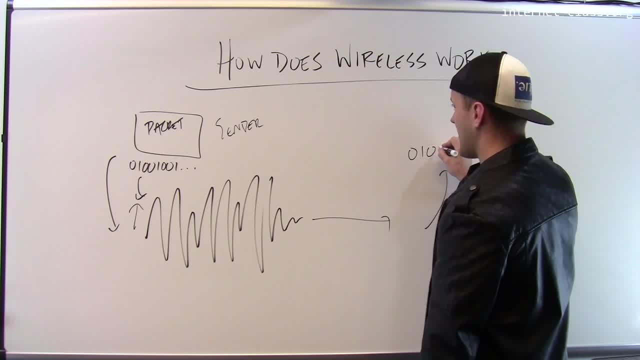 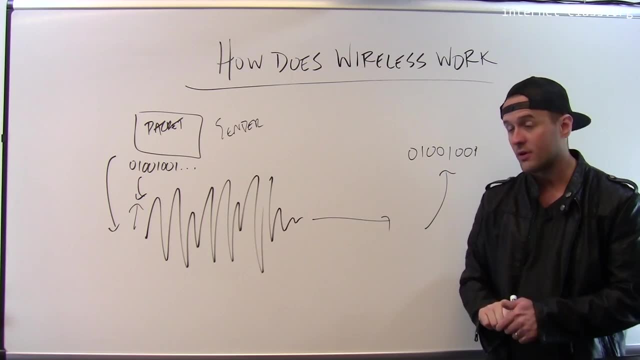 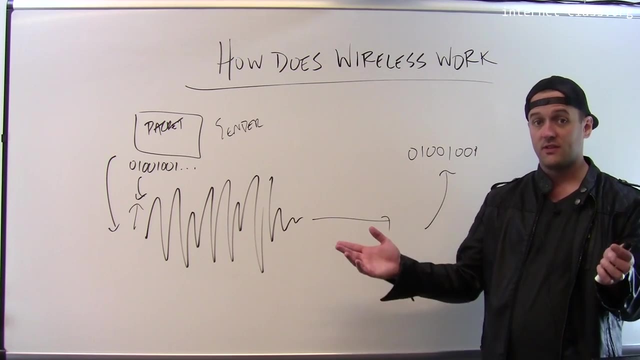 wave form and turn it back into the same series of ones and zeroes that the sender was trying to send. And what makes this difficult, of course, is that once this signal begins to propagate through free space, it's subject to interference from just things in the environment. 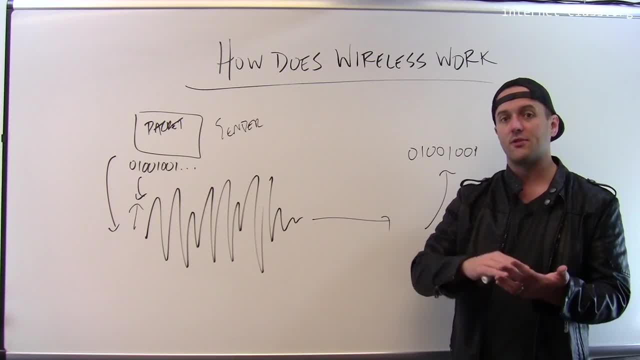 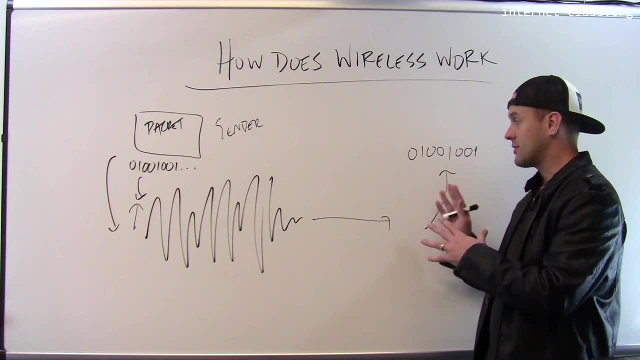 It tends to get weaker over time. So as the signal travels farther and farther, the amplitude of the signal diminishes. And there are also lots of other details in terms of how the receiver picks up the signal, But in general the receiver is not going to receive or not going to sense the exact